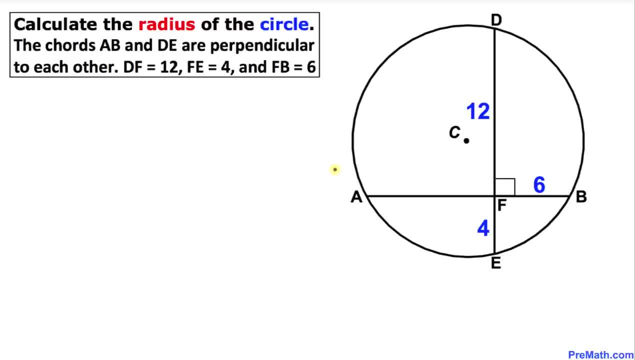 Welcome to PreMath. In this video tutorial, we are going to calculate the radius of the circle, as you can see in this figure. Moreover, the chords AB and DE are perpendicular to each other. DF is 12 units, FE is 4, and FB is 6.. 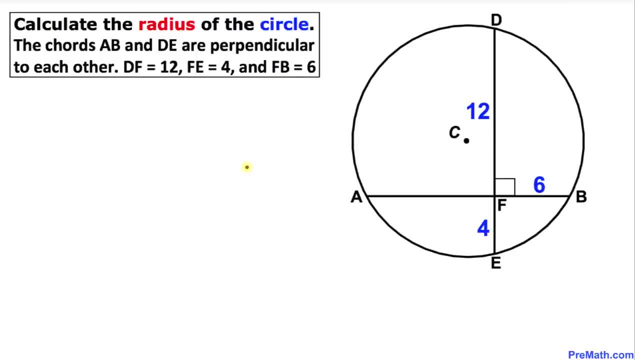 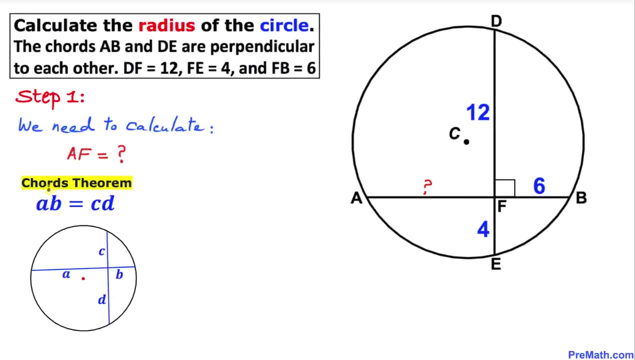 So let's go ahead and get started with our solution. And here's our very first step. We need to calculate this AF, part of the chord. We don't know the value. Let's go ahead and calculate this AF. Now. let's recall the intersecting chords theorem. 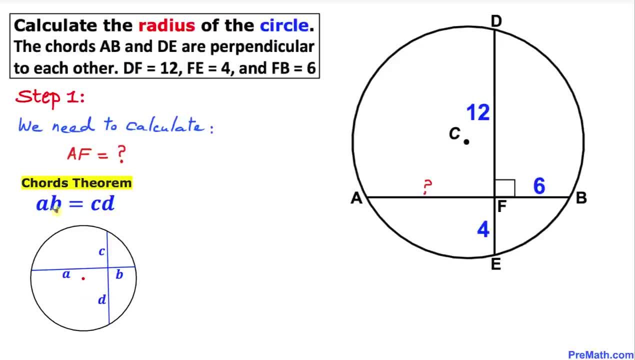 As you can see, two chords are intersecting each other. Then AB equals to CD. That means this A times B equal to C times D. Let's use this analogy to our this given figure. So that means this side is going to be an A, this B, this C and this D. 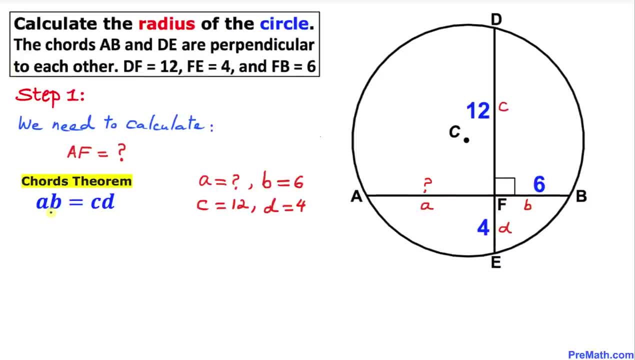 And we need to calculate A. Now let's go ahead and apply this theorem In our case. A, we don't know. B, in our case, is 6 equal to C, is 12 times D is 4.. So that is going to give us 6A equals to 48.. 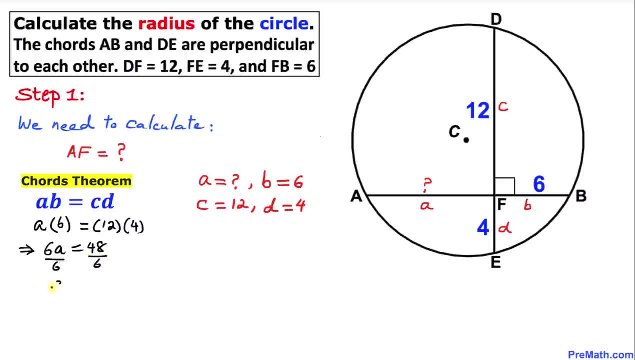 Let's divide both sides by 6. So A turns out to be 8.. So thus our A value turns out to be 8.. And we know that A is same as this AF part, So therefore AF equals to 8.. 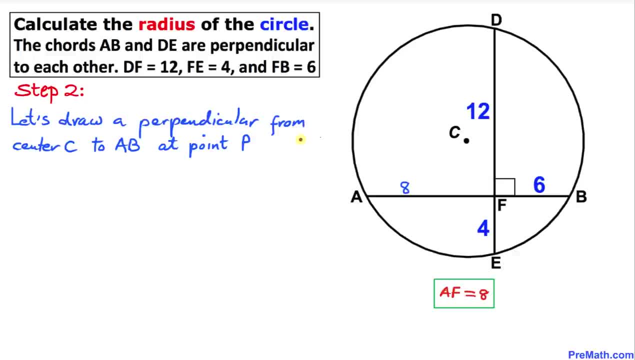 And here's our next step. Let's draw a perpendicular from this center C onto this chord AB. Let's go ahead and do this one. Let's draw a perpendicular over here. And this is a perpendicular, by the way, And this point A, I'm going to call it P. 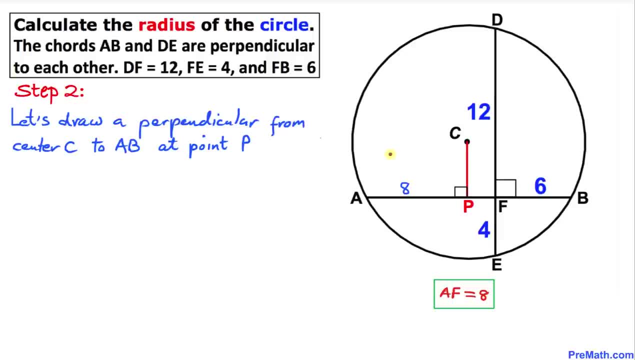 And here it is our nicer looking diagram. And here it is our nicer looking diagram. And here is our chord of a circle theorem: A radius perpendicular to a chord divides the chord into two equal parts. And here is our CP. This is our radius. 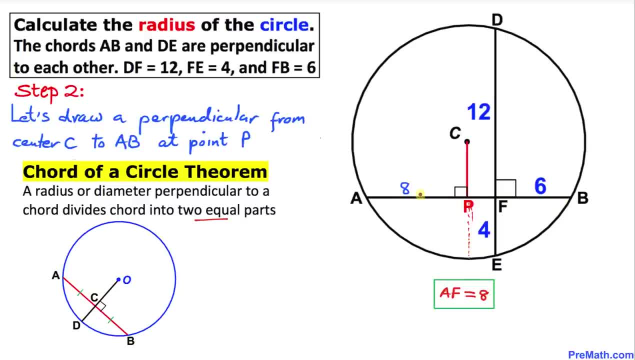 Okay, And this AP is a chord. That means it's going to divide this one into two parts. AP equals to PB, So therefore, AP equals to BP, And we also know that the total length of this AB is going to be 8 plus 6.. 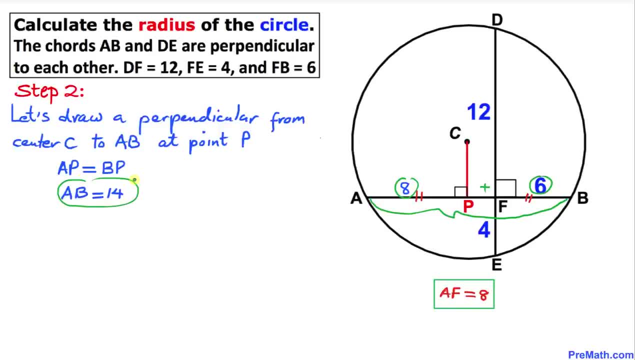 That is going to give us AB equals to 14.. And we also know that this AP distance is half of this AB. So we're going to divide 14, divided by 2.. Therefore, the length of AP turns out to be 7.. 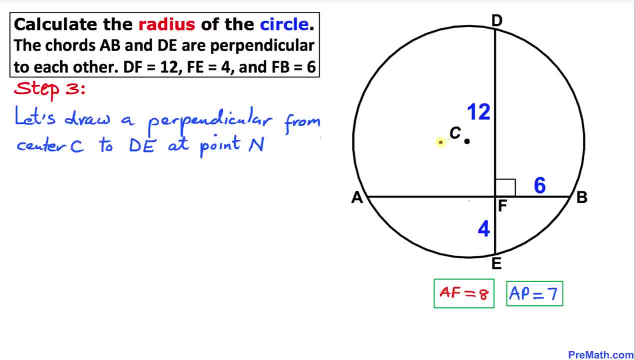 And here is our original figure. once again, And this time we are going to draw a perpendicular from this center to this line DE. Let's go ahead and draw the perpendicular over here, Somewhere here, And I'm going to call this point over here N. 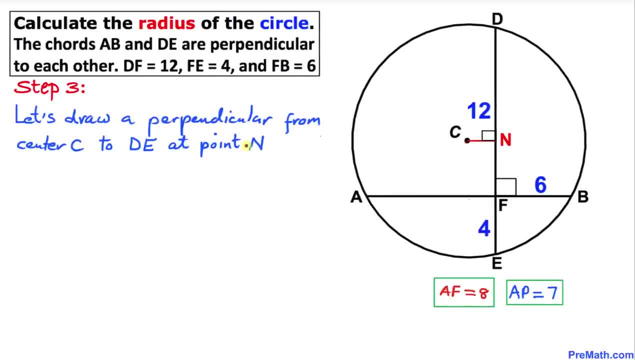 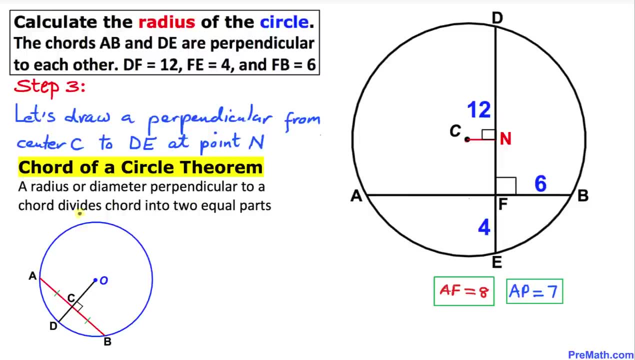 And here is our much nicer looking diagram. And now let's recall the chord of a circle. theorem once again: A radius perpendicular to a chord divides the chord into two equal parts. This time this CN, this is our radius And this DE is our chord. 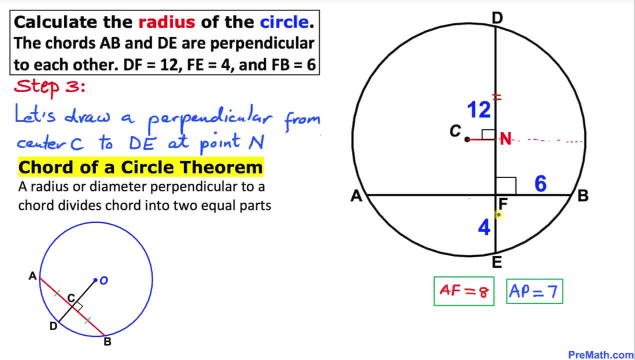 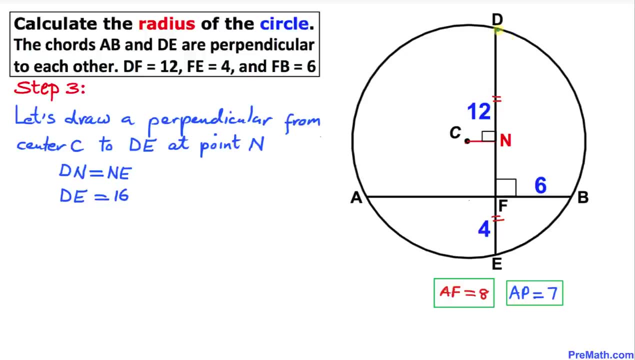 So then it's going to divide this chord into two parts. The first one is going to be DN and the other one is going to be NE. So therefore, we got DN equals to NE, And we also know that the total length of this DE is going to be 12 plus 4 is going to give us 16.. 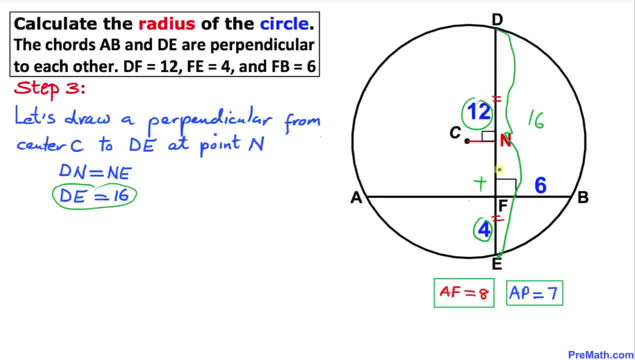 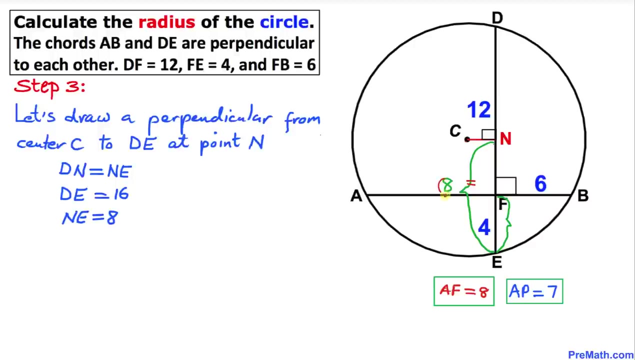 As you can see over here. And one more thing: This NE, this one, is the half of this DE. So we are going to divide 16 divided by 2. That means NE is going to be 8 units. So we know that NE is 8 units. 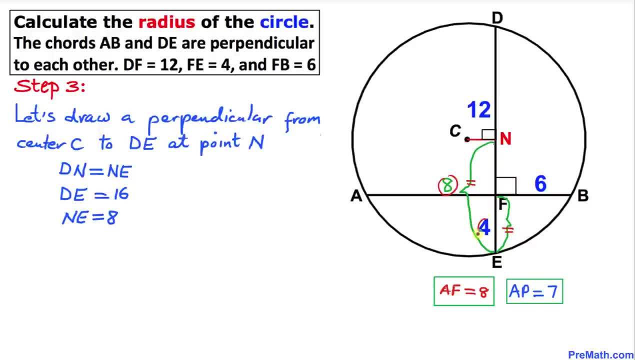 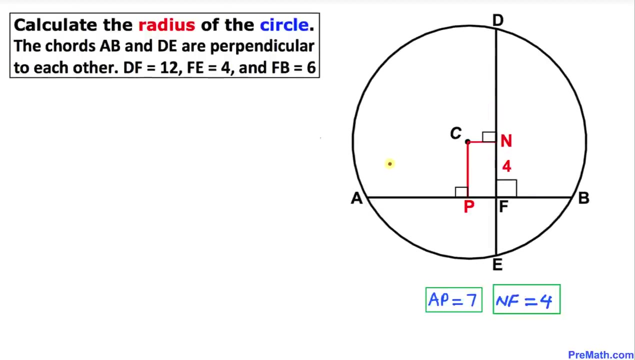 And we know that this FE is 4.. So then, this NF is going to be the difference: 8 minus 4 is going to be 4 units. So thus this NF turns out to be: this one is 4.. And here is our new figure, once I have put together two previous figures. 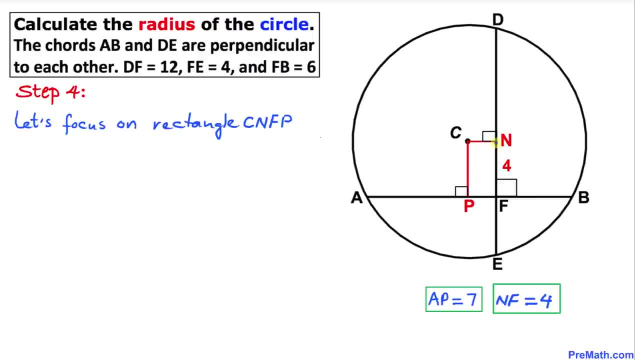 Now let's focus on this rectangle, CNFP. And here is the definition of rectangle. It has four angles, each measuring 90 degrees. The opposite sides of rectangle have same lengths and are parallel, So that means this side is going to have the same length as this one. 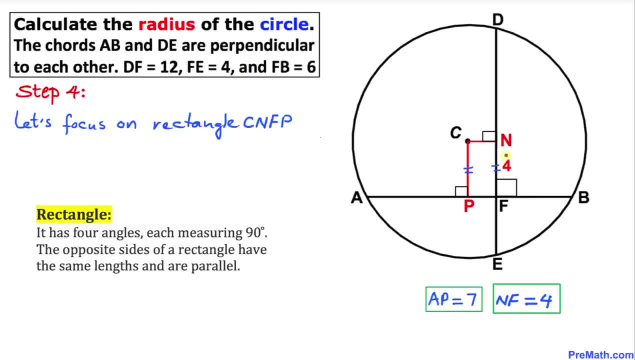 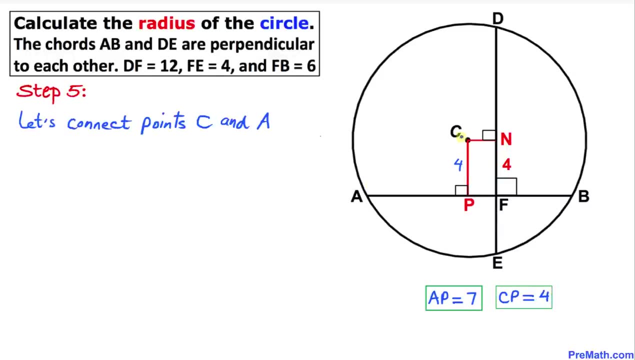 And they are parallel as well. And since this one is 4 units, So this CP is got to be 4 units as well. So thus our CP turns out to be 4.. And in this next step, let's go ahead and connect this point C and A. 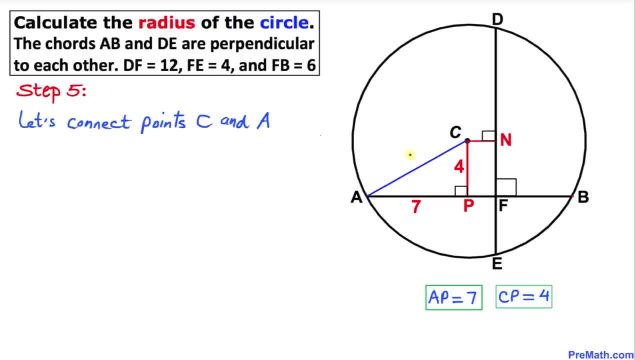 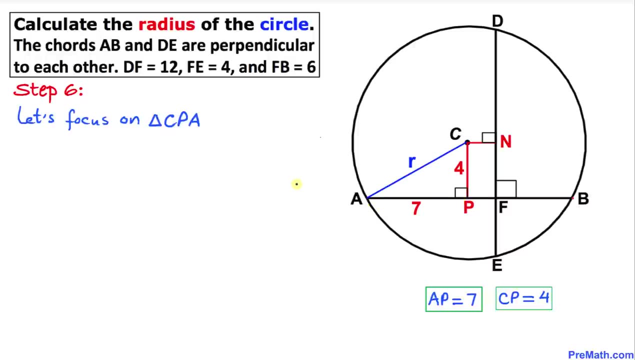 And here is our much nicer looking diagram And you can see that AC, this is our radius. I am going to call it R And here is our final step. Let's focus on this triangle, CPA, And since this is a right triangle, 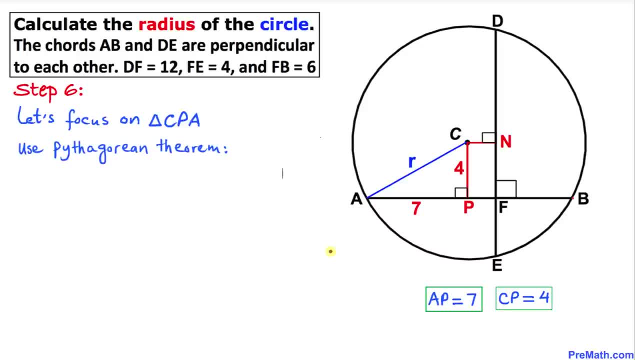 So we are going to use the Pythagorean theorem. And here is the Pythagorean theorem: A square plus B square equal to C square. In our case. I am going to call this side A, which is 7.. This side B, which is going to be 4..